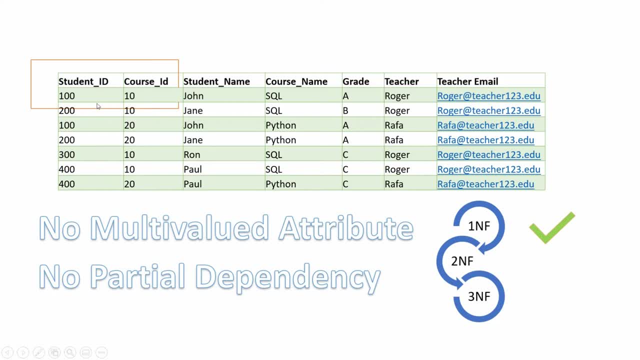 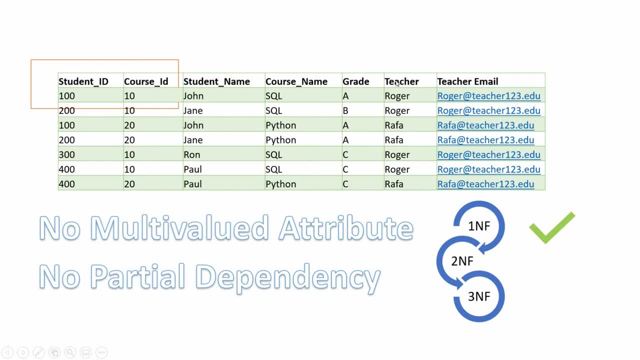 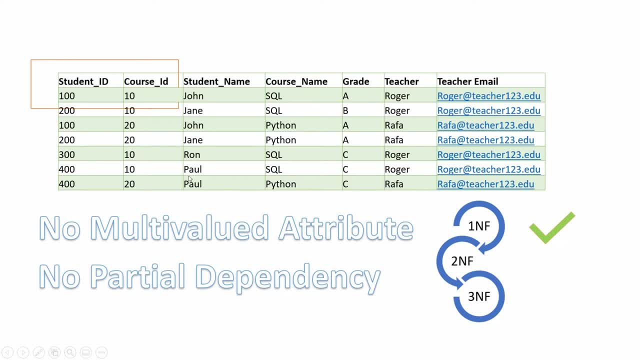 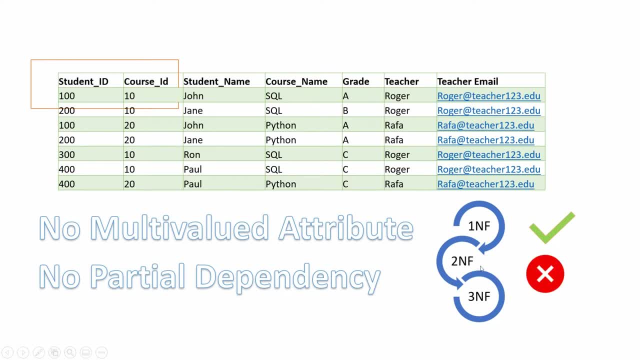 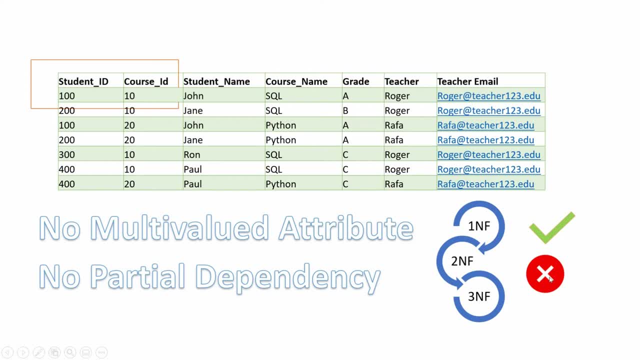 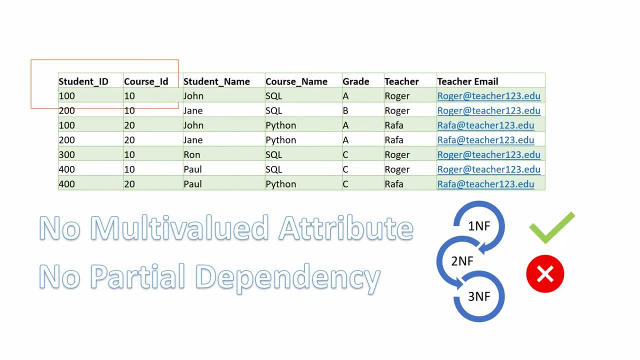 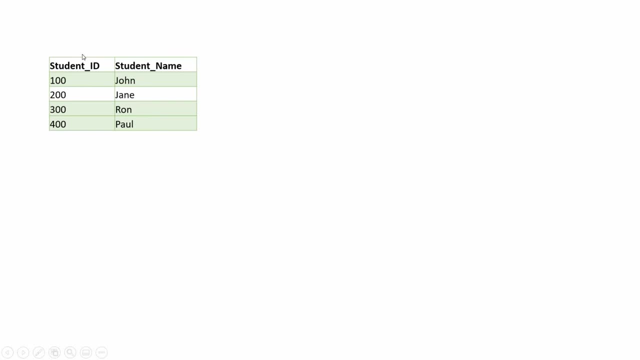 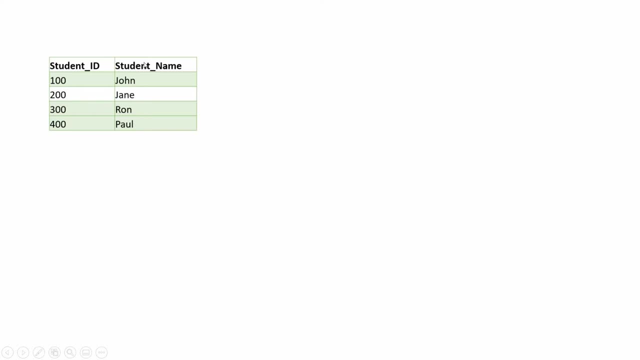 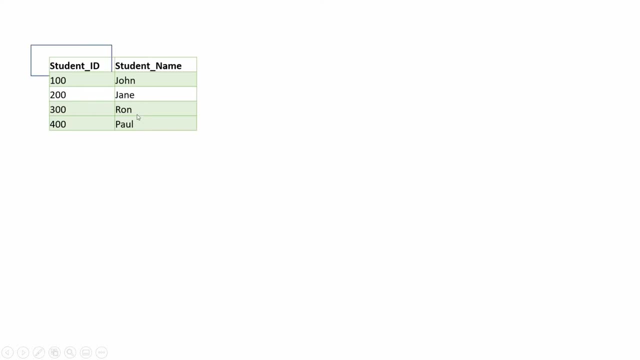 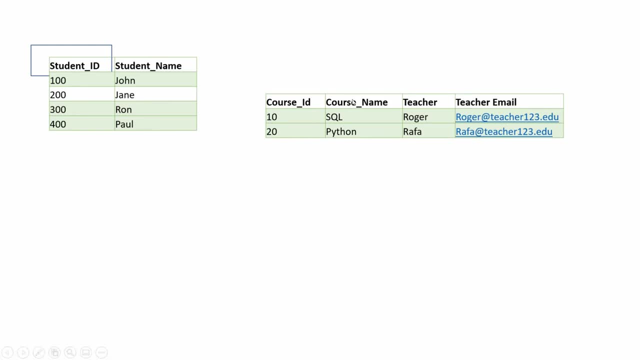 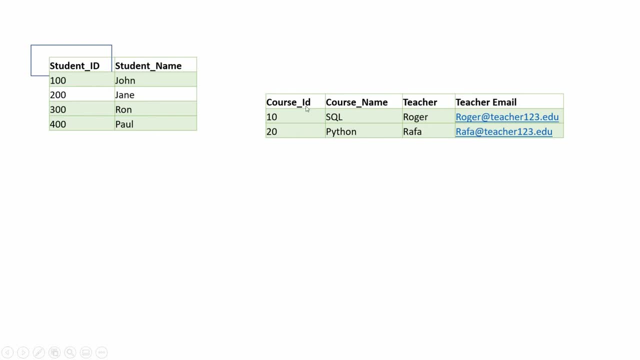 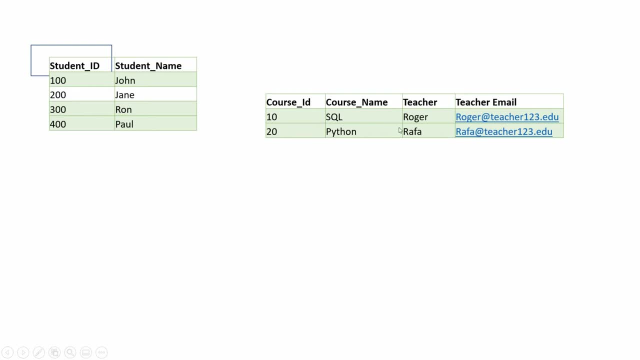 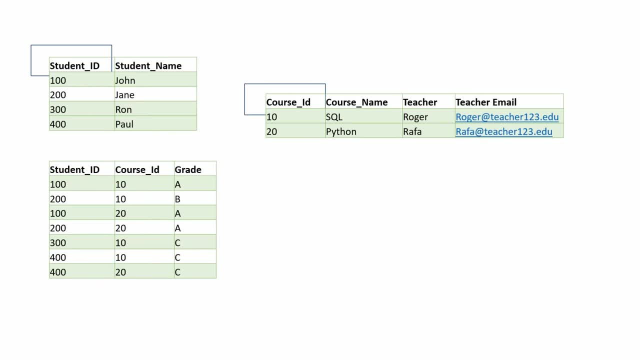 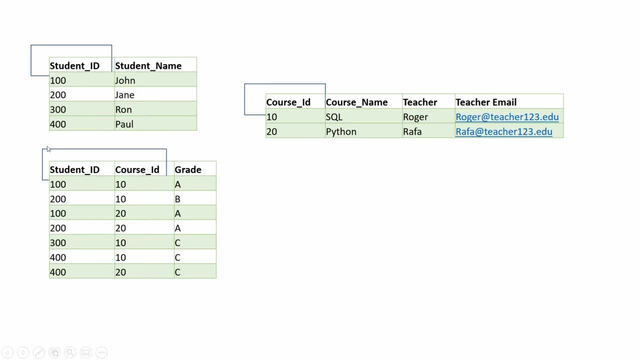 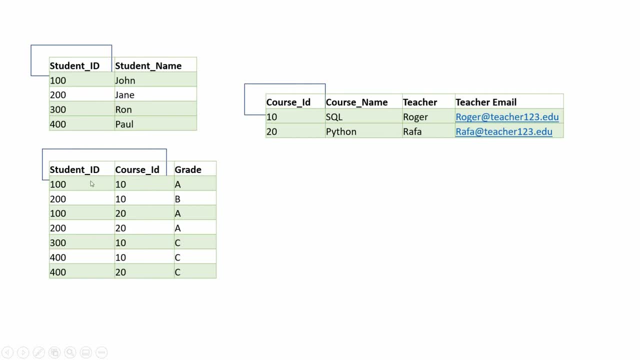 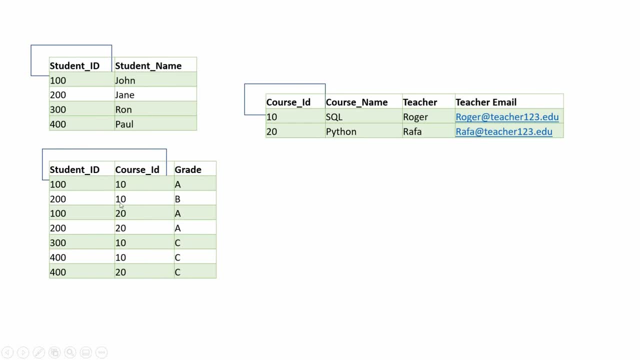 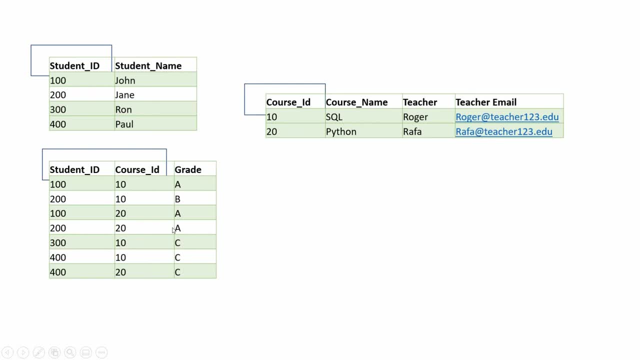 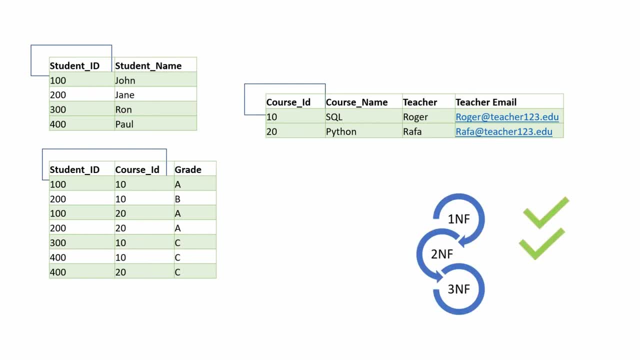 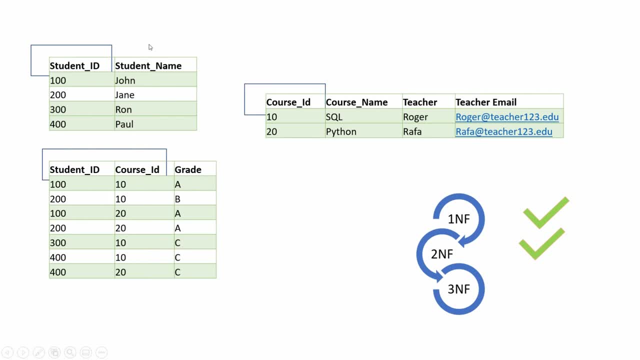 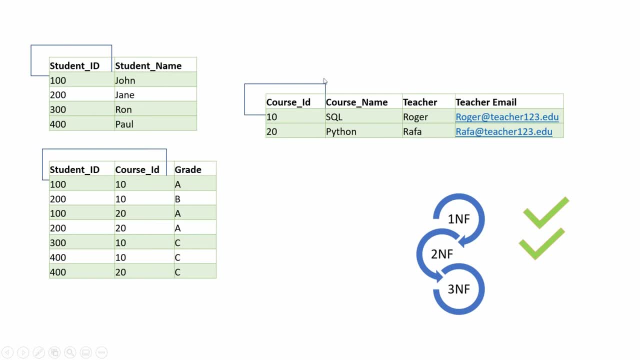 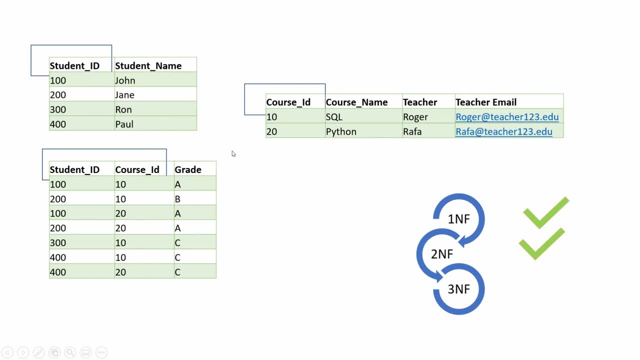 we have created these two tables and we have grade, which is dependent on both student ID and course ID, which is why we have created the third bridge table. now let's see if these tables are in third normal form as well. third normal form states that the table should be in second normal form and there should not. 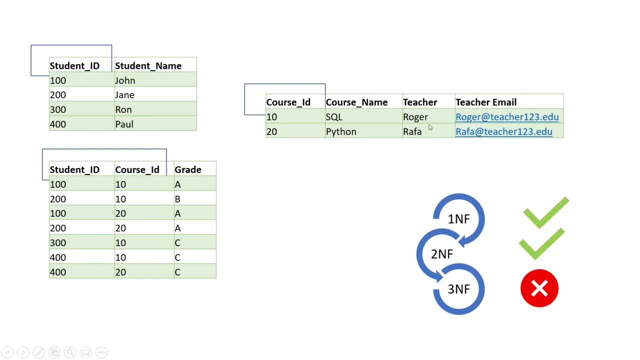 be any transitive dependency, that is, no non prime attribute should be dependent on any other non prime attribute of a table. this is violated for the course table. so this data set is in 2 NF but not in 3 NF, to make it third normal form. 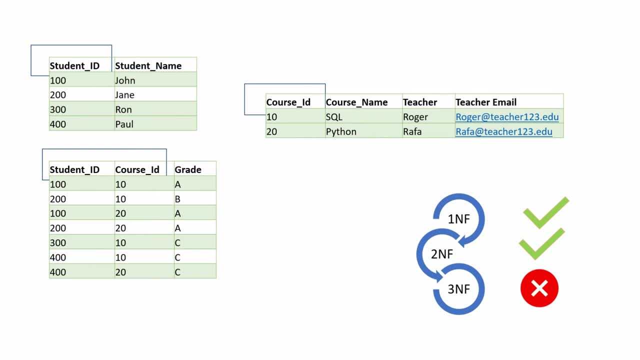 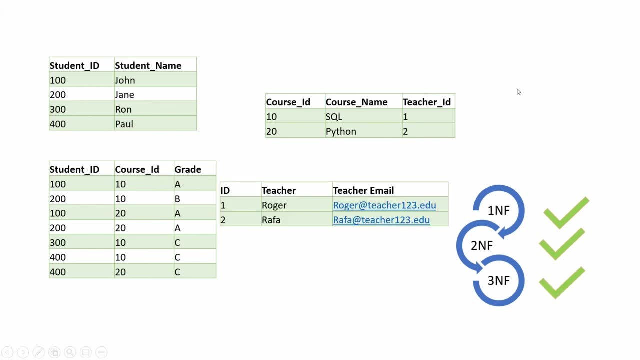 compliant. we need to break our course table into two separate data sets, like below. so a quick recap: if you have a denormalized data set and you have to make it third normal form compliant, you have to ensure first that it is in first normal form and then you have to make it second normal form compliant. and finally, 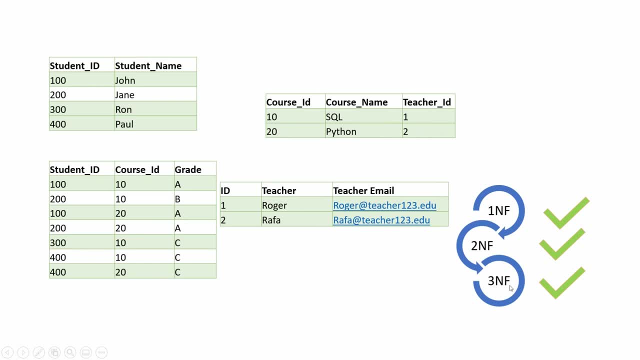 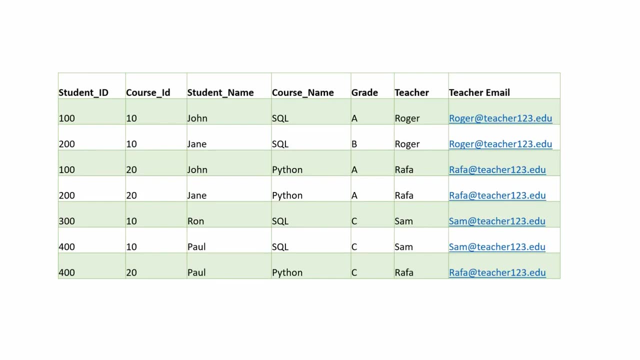 you need to ensure that it follows all the property to stay third normal form compliant. now here is the same data set with a slight change. earlier only one teacher could teach a course, but here both roger and sam are teaching the same subject, sql. can you make this dataset in third normal form? post your solution in the comment section. 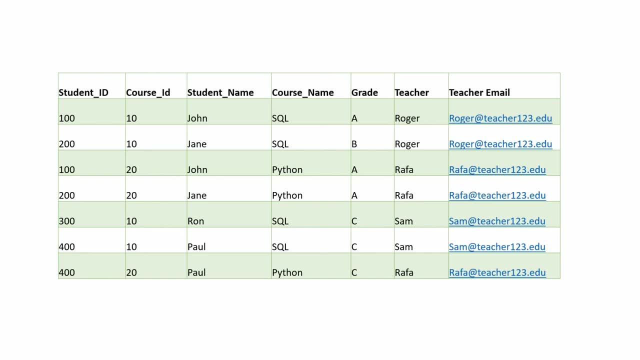 if you require any clarifications, do let me know. i will be more than happy to assist, and please subscribe if you have not done already, and don't forget to press the bell icon so that you get a notification as soon as i publish a new video. thanks a lot, guys, for. 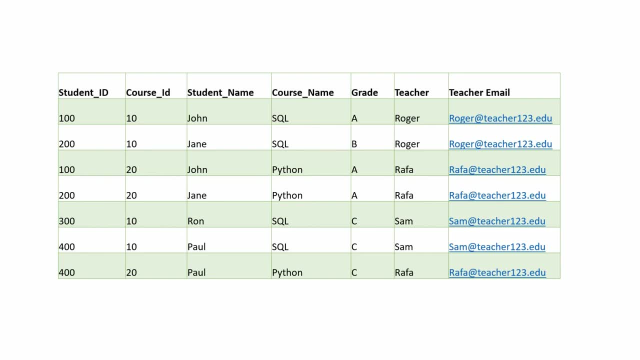 watching this video. your support is my motivation. 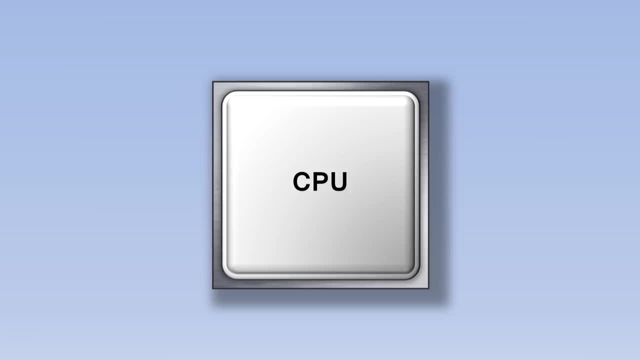 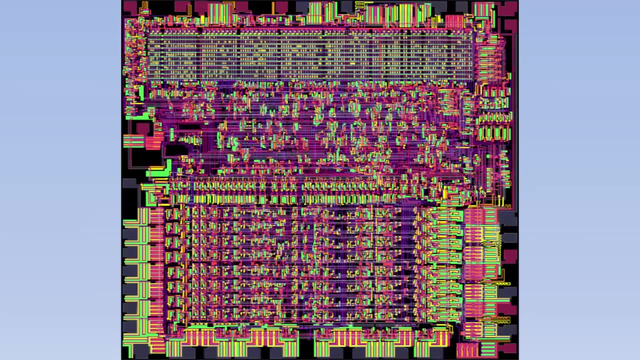 The CPU, short for Central Processing Unit, is like the brain of the computer, and once you understand how it works, you'll understand the computer as well. Let's remove the cover of the CPU and zoom in to see what happens inside. There are lots of different wires carrying information around the CPU. 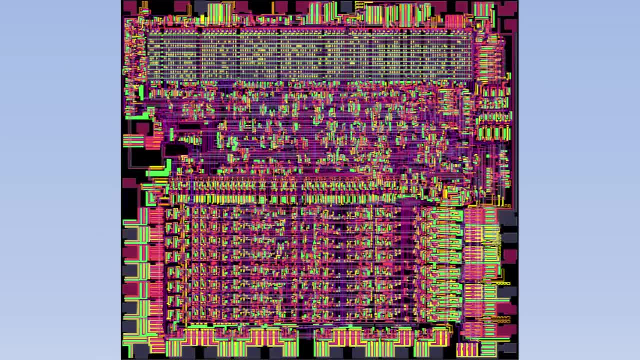 This particular CPU is called the 6502 and was used in computers like the Apple II and the Commodore 64, as well as in the original Nintendo Entertainment System. This simulation of the 6502 can be found online at visual6502.org. 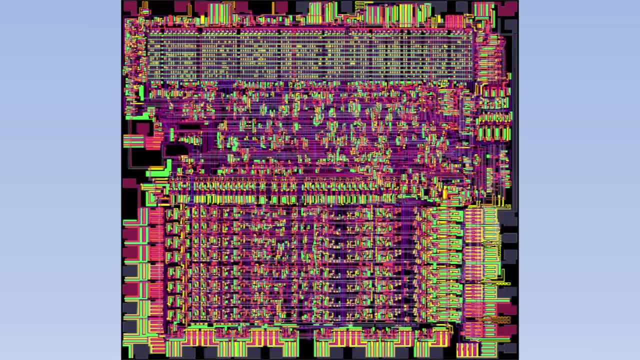 In every CPU there is a particular wire that turns on and off at a steady rate to help keep everything in sync. That wire is called the clock, and the clock in this simulation is turning on about twice a second. Modern CPUs are measured in gigahertz- giga meaning billion, and hertz meaning times per second. 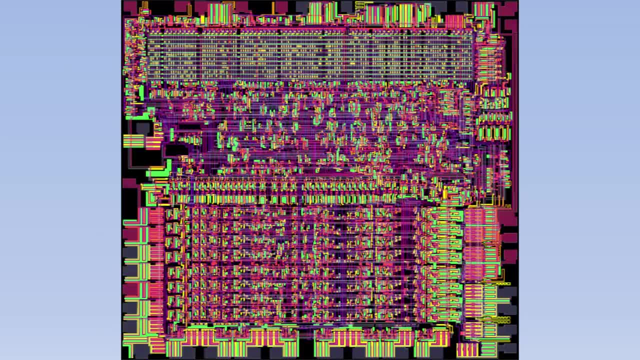 So the clock in modern CPUs turns on several billion times per second. That speed is what allows CPUs to do things like this. They can do very complicated things very quickly. However, what the CPU does during each clock tick is actually very simple and something we'll look at more in this video.